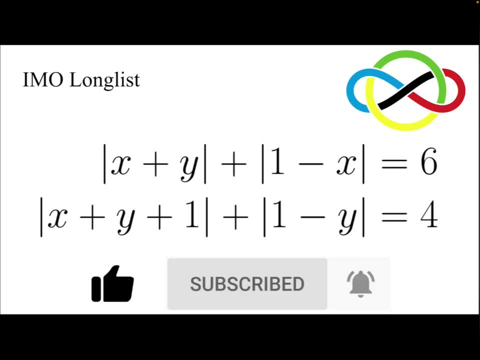 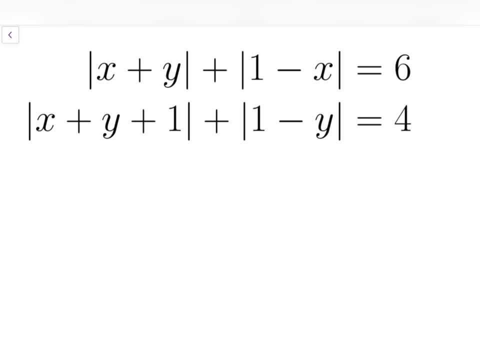 give a like, subscribe to my channel and turn on post notifications. The usual way to solve equations that involve absolute values is to divide into a few cases, For example for 1 minus x or 1 minus y, and I will split into cases. say x is less than 1.. 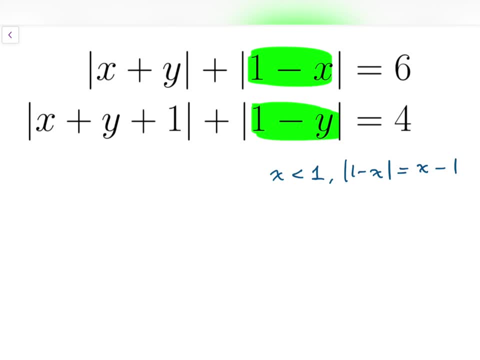 Then I can just remove the sign and replace it by the expression x minus 1.. Otherwise I will just keep it The same or wait. it seems I mixed them up. For this case I should be keeping that inside, because 1 minus x is then positive, While for the other case that is rewriting as x. 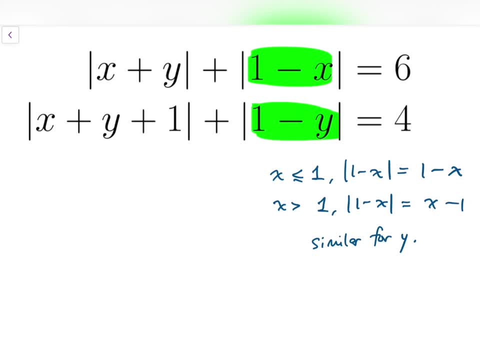 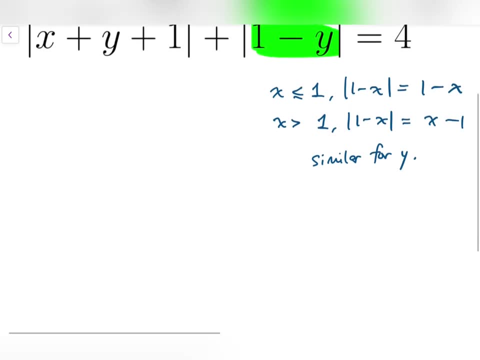 minus 1, as similar for y. That's the usual approach, but this time it's too complicated, because if you're trying to look at the expression and the distribution as a whole, then you're more likely to get a false look at it with a graph and we have something like this: 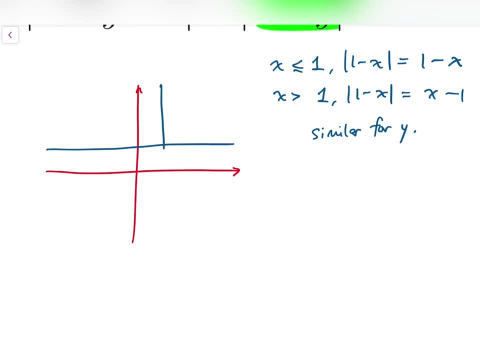 so here are the axis. we have x and y equals one that look like this: as for the other two expressions, x plus y and x plus y plus one, can be divided into, can be interpreted by this graph, which are: x plus y equals zero and x plus y plus one equals zero, respectively. 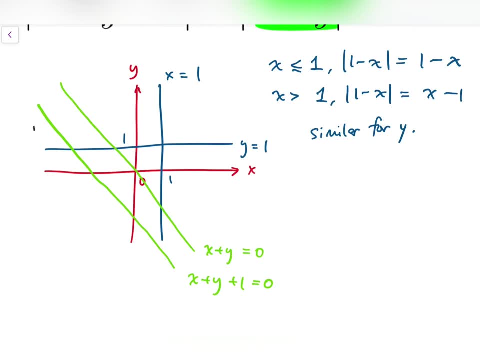 so then, the usual approach would be to consider each of these regions separated by the green lines and the blue lines, and then we have a graph, but this is extremely complicated, so what I'm going to do to solve this problem will be to focus on the value that x plus y takes. 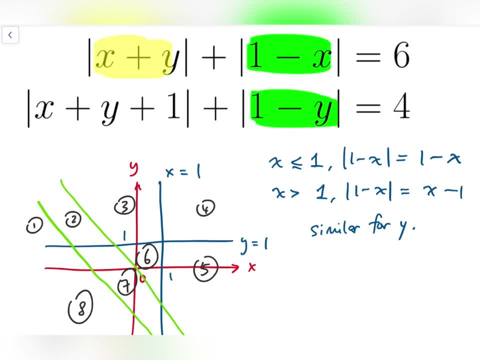 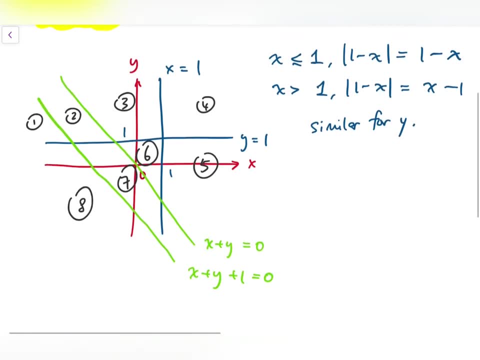 because that appears in both equations, so I'm going to focus on this instead. a graphical way to interpret this would be to shift this to the right, so we can see that we have a graph and we have a green line along the same direction. so then x plus y will take different values. 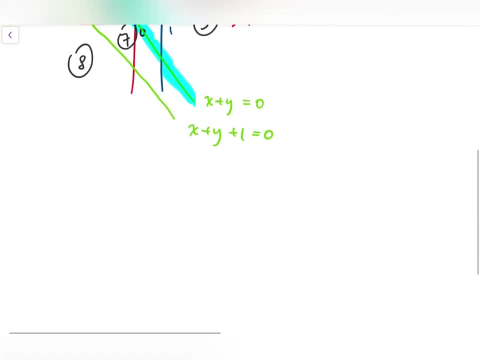 and then we will see what kind of solutions we can find along each of these lines. to do this, I'm going to let k to be x plus y and looking at the equations so far we have. for each equation we have 2 absolute values added together. 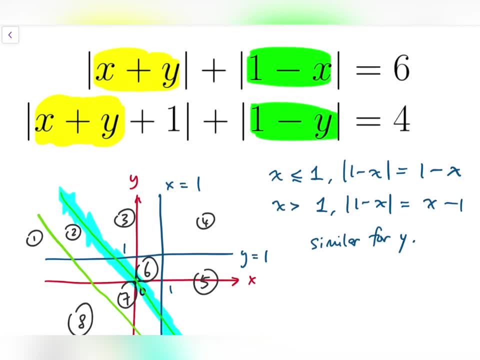 to be equal to some positive integer, so to I'm going to first establish a bound on x plus y. to do this, I'm going to say that, apart from the terms that contain x plus y, these absolute values must be non-negative. that's by definition of the absolute value. so from this we can assume that the terms which are present in terms of x and y that he is going to defined in this type of equation mean that e is the absolute value of e that h and r would be also equal to. so these absolute value must be non-negative. that's by definition of the absolute value. 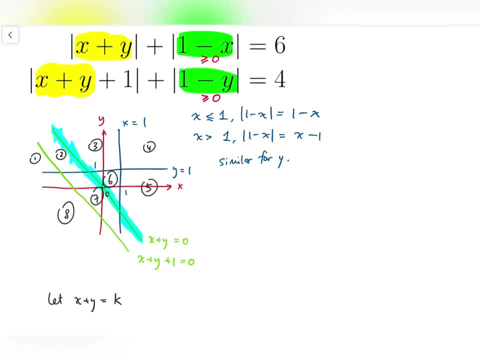 can say that, on one hand, we have the absolute value of x plus y to be at most 6- because this expression is added by something non-negative- to be equal to 6 and, at the same time, if it's x plus y plus 1, the absolute value is less than. 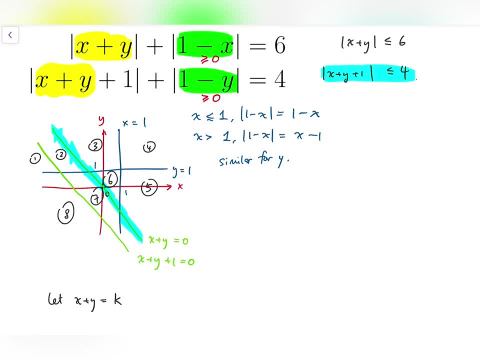 equal to 4 and apparently this will give us a more accurate bound, and let's proceed from this. So, removing the absolute value sign, we have x plus 5 plus 1 to be between minus 4 and 4, and x plus y is now between minus 5 and 3.. So 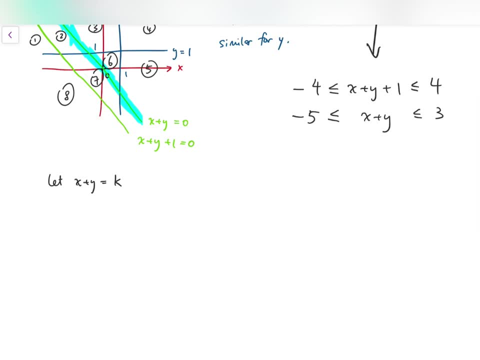 let's see what happens when x plus y takes each of these values. Since the expressions that contain x plus y are absolute value of x plus y and the absolute value of x plus y plus 1, they changed signs as in either from minus to plus, when x plus y takes either. 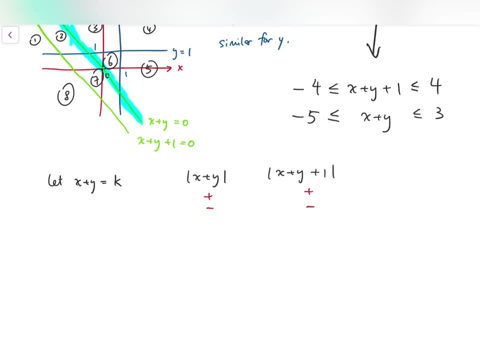 less than or larger than minus 1, or less than or larger than minus 2.. We might larger than 0. So I will treat minus 1 and 0 as some boundaries to split into cases for us. to split into cases, which means that I'm going to consider: 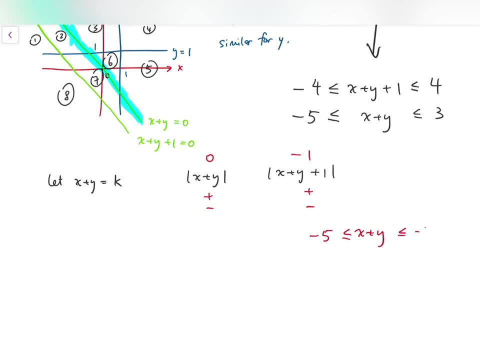 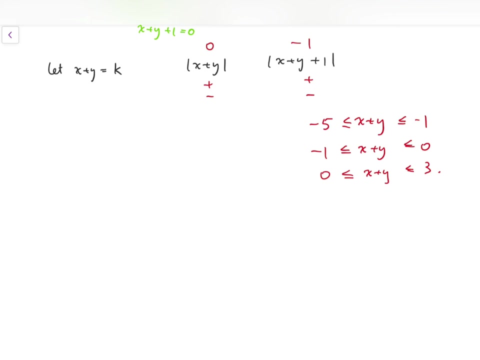 separately on x plus y, between minus 5 and minus 1, minus 1 and 0, and 0 to 3.. So here we have three cases. We know that we are replacing x plus y by k, so absolute value of k. 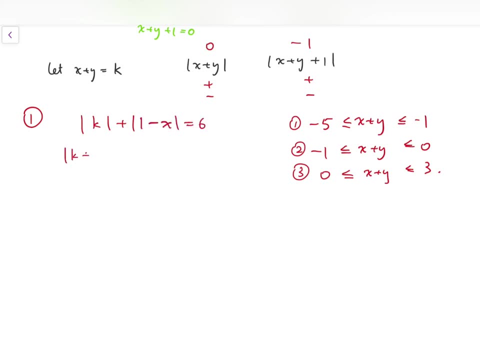 plus 0 is 0.. Absolute value of 1 minus x equals x, and k plus 1, absolute value plus absolute value of 1 minus y equals 4.. So now, under this case, both k and k plus 1 are still. 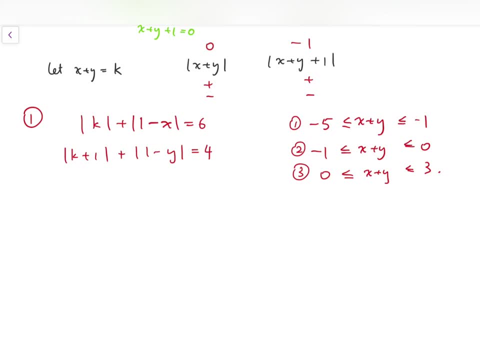 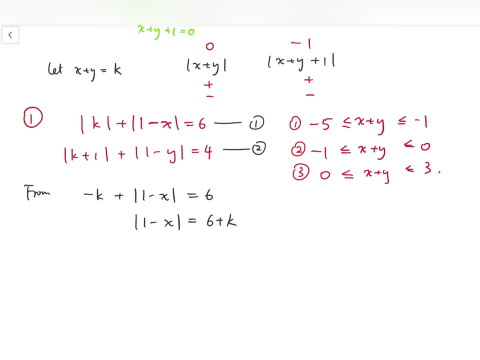 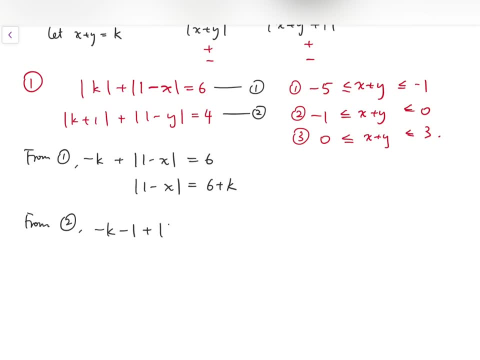 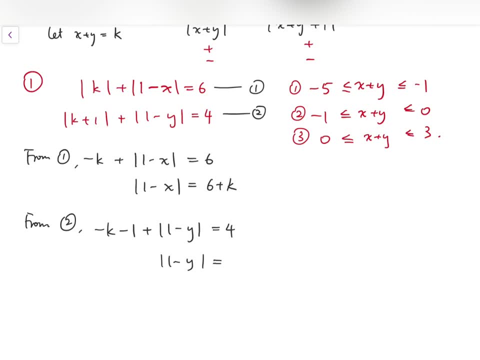 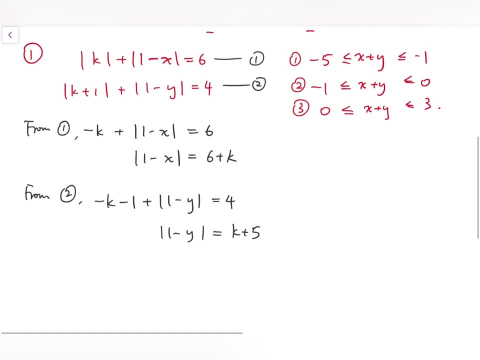 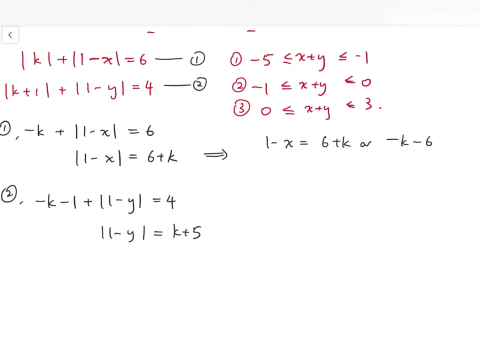 So now from the first equation I'll have absolute value of 1 minus x equals 6 plus k. So now from the first equation I'll have absolute value of 1 minus x equals 6 plus k. So now from the first equation I'll have absolute value of 1 minus x equals 6 plus. 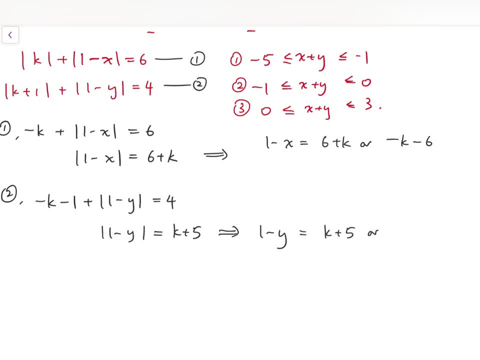 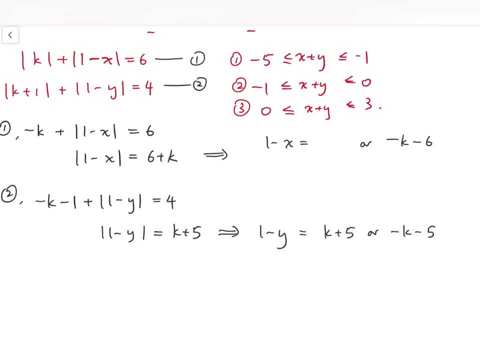 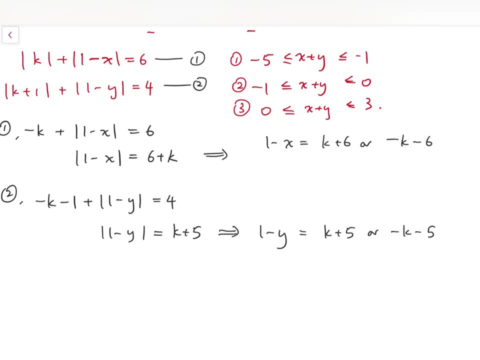 So now from the first equation I'll have absolute value of 1 minus x equals 6 plus k. So now from the first equation I'll have absolute value of 1 minus x equals 6 plus k. So now from the first equation I'll have absolute value of 1 minus x equals 6 plus. 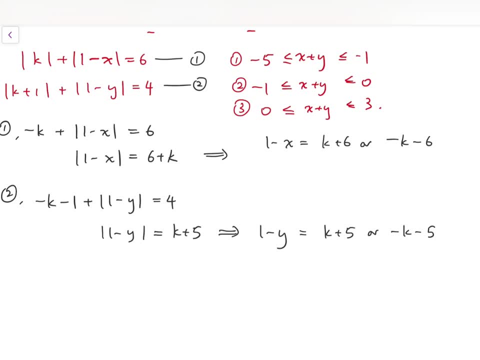 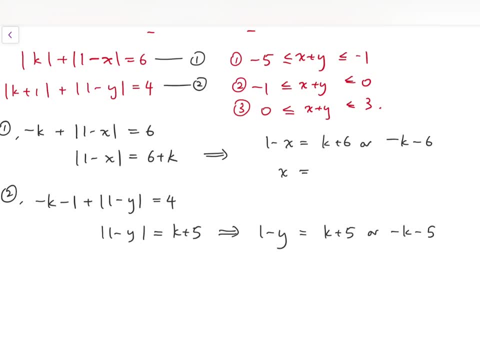 So now from the first equation I'll have absolute value of 1 minus x equals 6 plus k. So now from the first equation I'll have absolute value of 1 minus x equals 6 plus k. So now from the first equation I'll have absolute value of 1 minus x equals 6 plus. 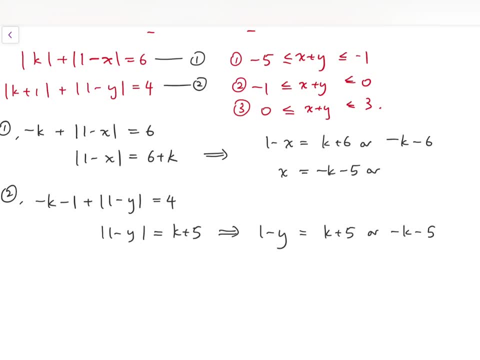 k From X, we have either minus k minus 5 or k plus 7.. And for d we have either minus k minus 4 or k plus 6.. So now we have these four possibilities: WeSpid or Db. 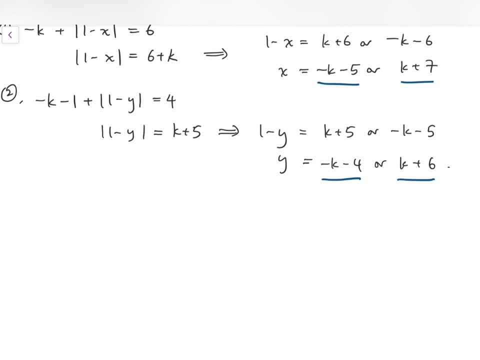 Then I'm going to add them and replace x plus y by k. To do this, x plus y takes four possible values, so it's either 1 with 1, which means minus 2k, minus 9, or taking the first possible value for x and the second possible value for y. 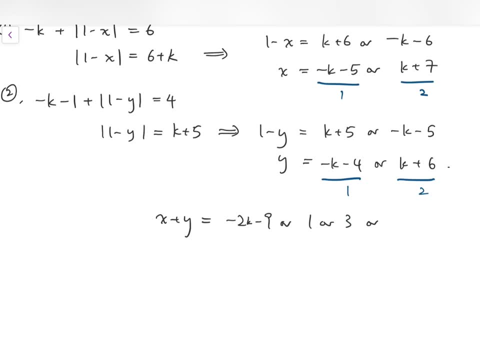 or reversing the order. then I will have either 1 or 3.. And lastly, for the last case, I will just add k plus 7 and k plus 6, which is 2k plus 13.. Okay, And this sum is equal to k, so we can solve for k. 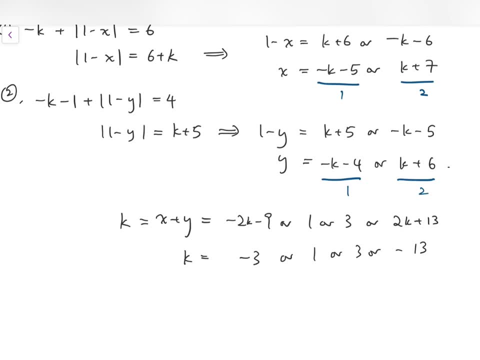 So it's either minus 3 or 1, or 3, or minus 13.. And you can see that because I've restricted k to be between minus 5 and minus 1, so this is the only possible case, which means k is minus 3.. 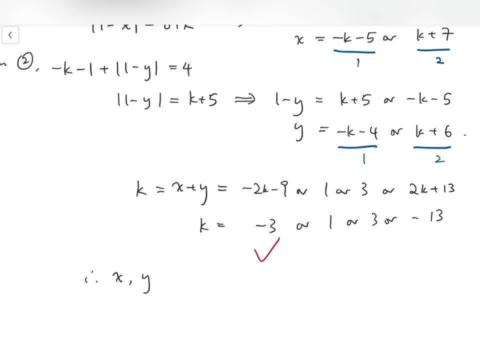 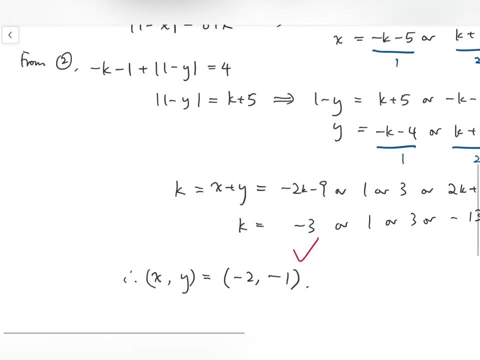 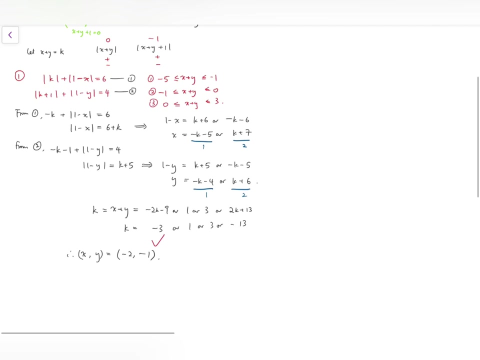 So then from this we can tell that therefore, x and y should be 3 minus 5,, which is minus 2, and y is 3 minus 4,, which is minus 1.. So now, from this case we have one pair of solution. 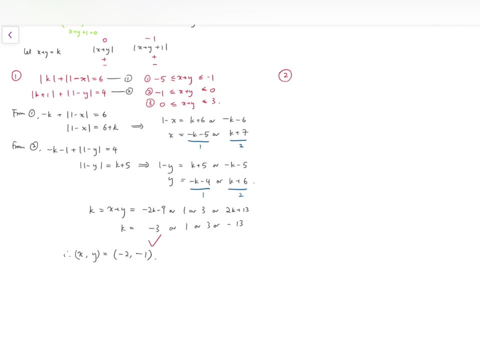 Now I'm going to do the same for the other two cases. I'm just going to zoom that out so you can see that more clearly. Okay, Now for the second case. I've assumed that k is between minus 1 and 0. 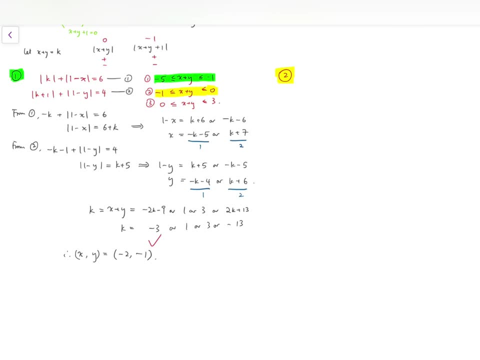 Now- this time it's a bit different- is that for the system that we're given, k is still negative. so for the first equation I will still write it as minus k plus the absolute value of 1 minus x equals 6.. 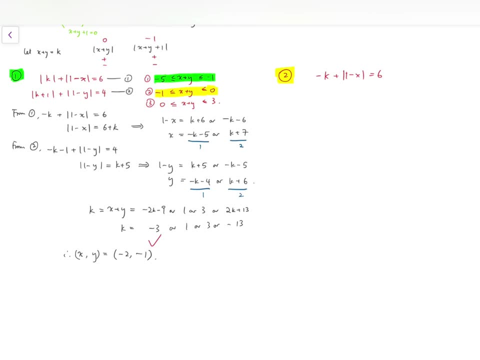 Okay, Now for the second equation. now k plus 1 becomes positive because it's between 0 and 1.. So I'm not going to add a minus sign at the front of it, just remove the absolute value. Now we have these two equations. 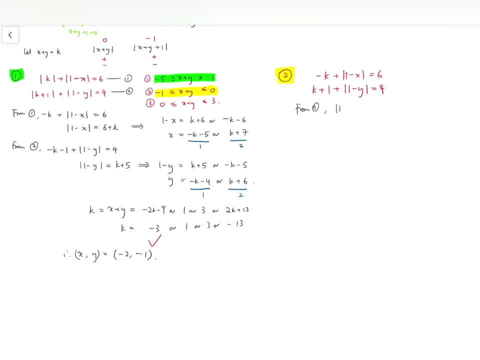 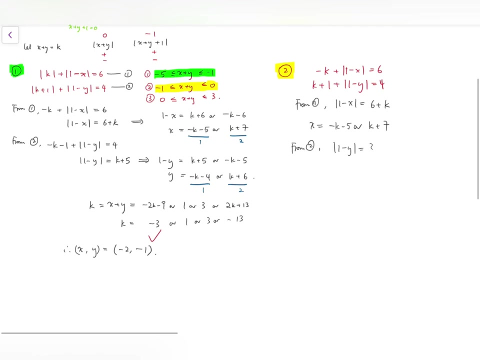 So now I'm using a similar argument. It will look like this, Just put it like this: times k: Okay, And the next equation we're going to follow is educators. I'm going to write this here, or we could go click here if you want to do that. you. 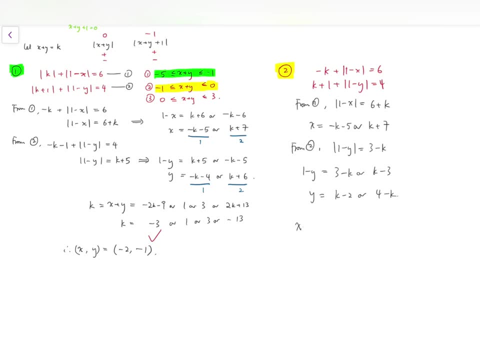 can click on it. Alright, See, we have these cases again, So now again I'll add them up. I have either minus 7, and then minus 2k minus 1, and then 2k plus 5,. 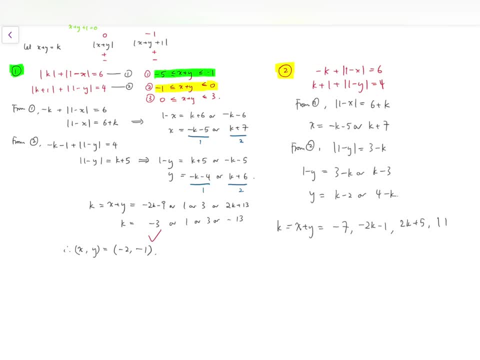 and at last I have 11. And they are just equal to k, So solving each of them. only the second case is correct: k is minus 1. third, because I've assumed that k is between minus 1 and 0.. 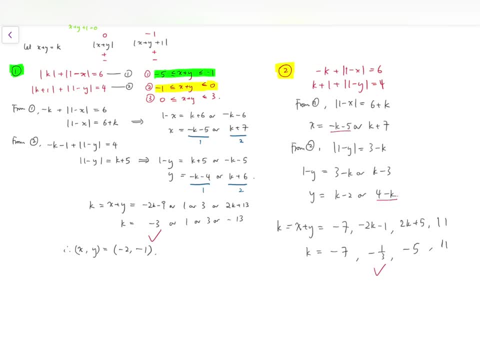 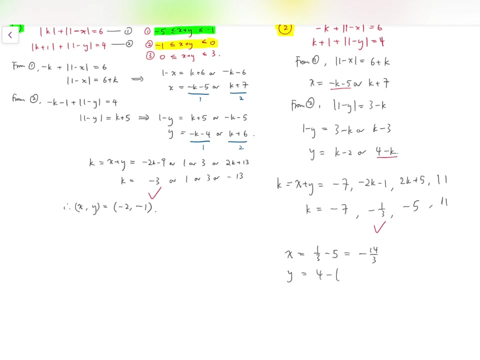 So from this this is actually taken from minus k minus 5 and 4 minus k. So then that means x equals 1 third, minus 5 equals minus 14,, 14 over 3, and y equals 4 minus negative 1 third. 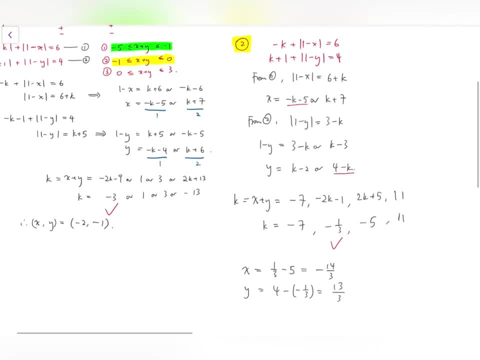 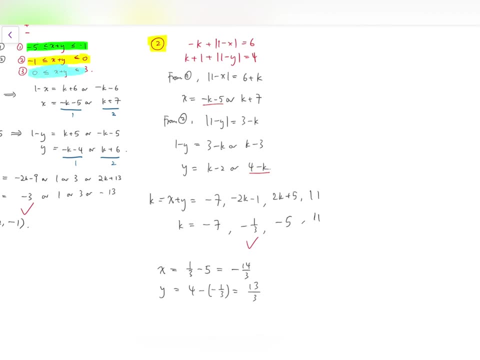 and that's 13 over 3.. So that's the second pair of solutions. Lastly, I'm going to settle the third case, which is when x plus y is between 0 and 3.. Now for this case. both k and k plus 1 are now positive.